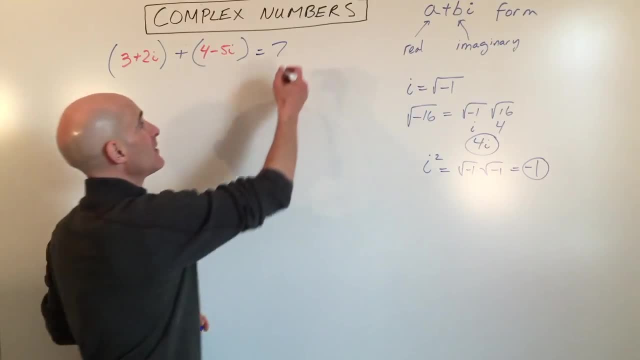 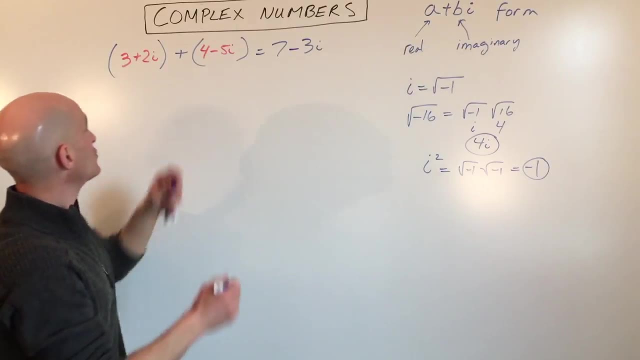 X, Y or Z, 2i plus negative 5i is negative 3i and that's it. that's an, a plus bi form, that standard form. now say you wanted to subtract the two complex numbers 3 plus 2i minus 4 minus 5i. same idea, you're just subtracting 3 minus 4. 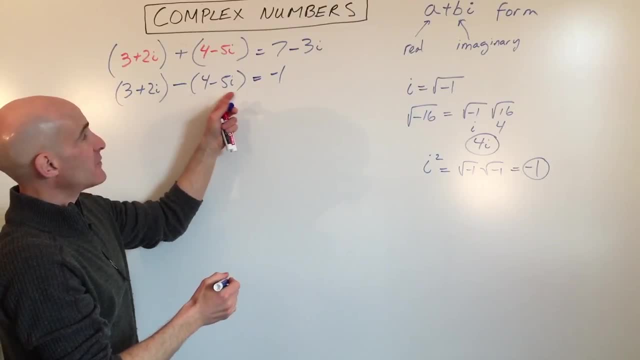 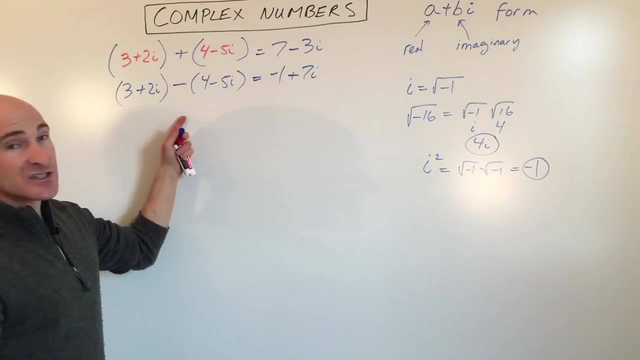 which equals negative 1, 2i minus a negative 5i is like adding 5i 2, negatives become a positive, so that's going to be 7i. now let's take a look at multiplication. so 3 plus 2i times 4 minus 5i, here you've got a binomial. 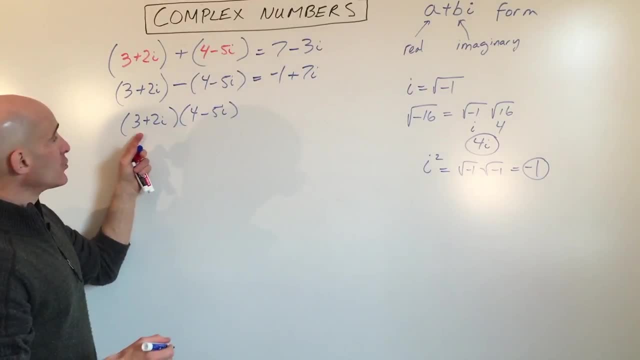 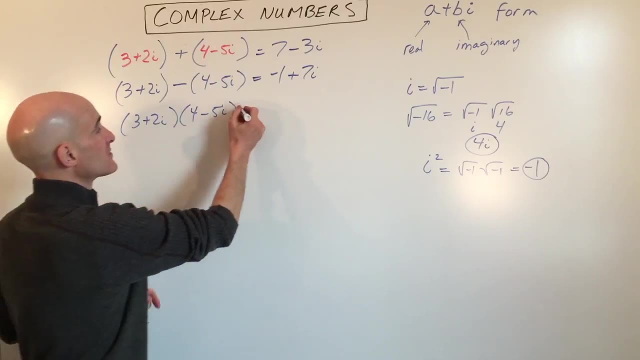 binomial times a binomial. you can FOIL, you can do the distributive property, however you like to work with a binomial times a binomial. so we're going to do the FOIL. first terms gives us the FOIL and then the FOIL gives us the 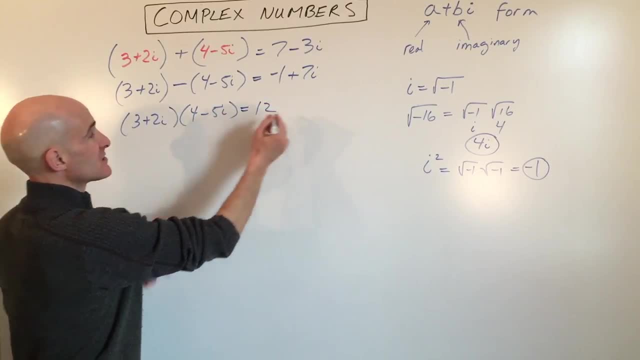 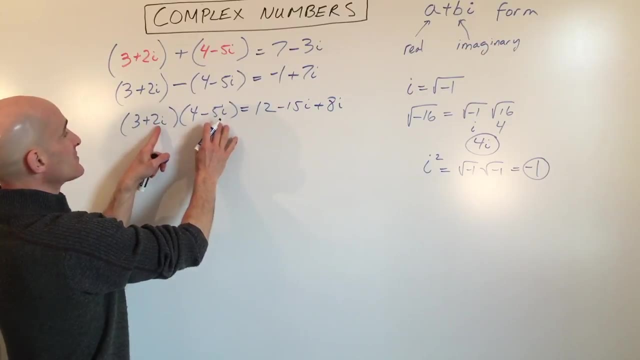 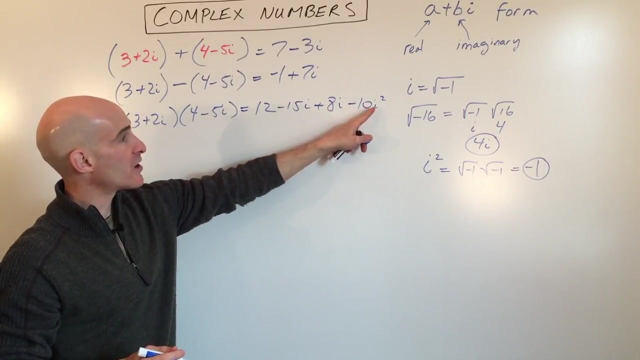 FOIL. innライfer terms gives us 12. outer terms gives us negative 15i. inner terms gives us 8i. and then the last terms gives us negative 10i. squared okay, because I times I isied two 77 corridor in the middle. remember I squared equals. 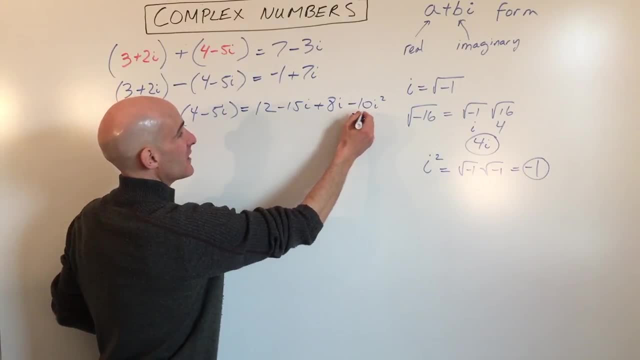 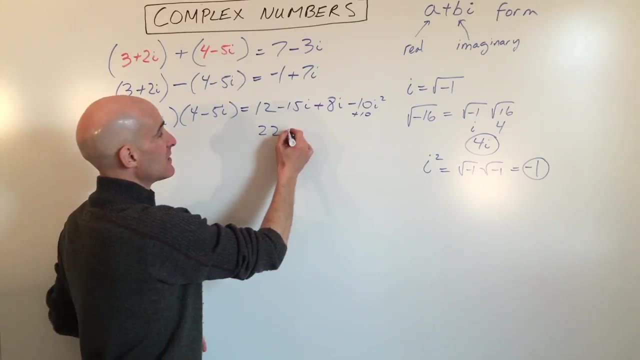 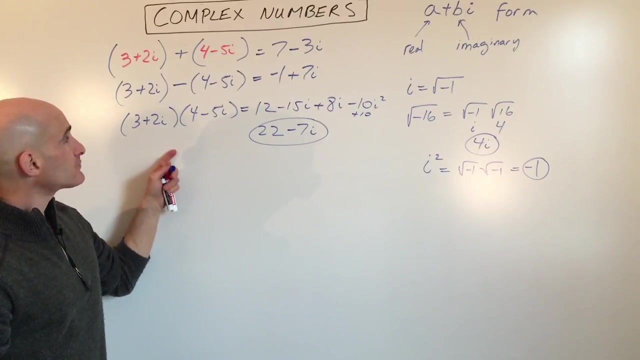 negative 1. so this is negative 1 times negative. 10 is positive 10. okay, so 12 plus 10 is 22 plus 8i is negative 7i. so that's these two complex numbers multiplied together, and then the last one we're going to talk about is dividing, so 3 plus 2i. 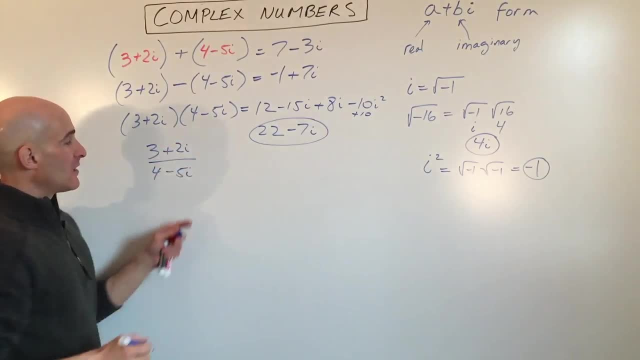 divided by 4 minus 5i. now you don't want i in the denominator. that's considered improper. so how do we get rid of the i in the denominator? you probably remember working with radicals and square roots and what we did there when we had a. 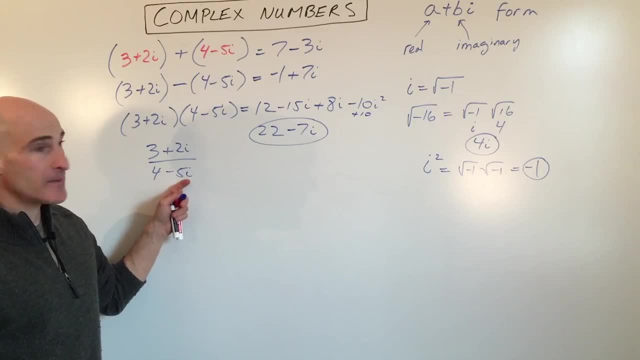 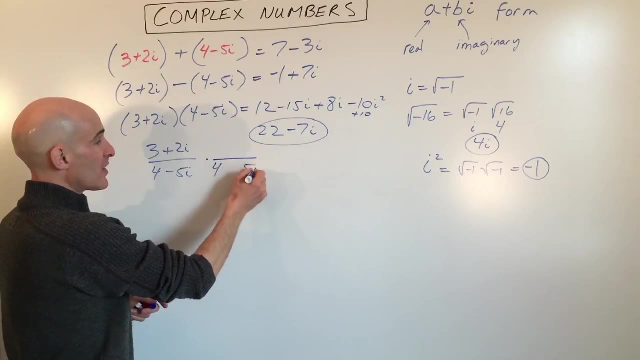 binomial two terms in the denominator is we multiplied by the conjugate? here we're going to do a similar thing. it's we're multiplying by the complex conjugate, because this is a complex number. you're going to write these same two terms, but instead of minus, you're going to put a plus here. if this was, 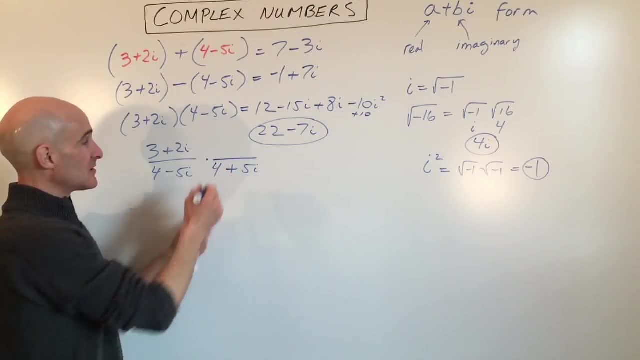 adding. you'd make this subtracting, so you just make these signs the opposite, of course. whatever you multiply the denominator by, you want to multiply the numerator by? okay, because this is really like one one times. anything doesn't change the value of this fraction, just changes the way that it looks. and 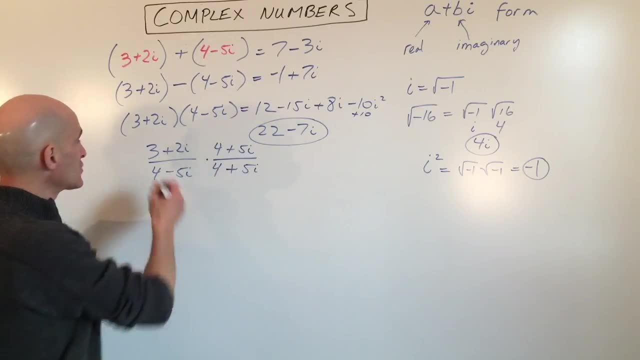 puts it into a nicer, neater standard form. so let's go ahead and do this. we're going to multiply these together. let's do the denominator first. we have 4 times 4, which is 16, negative 20i and positive 20i. those cancel and the last terms gives. 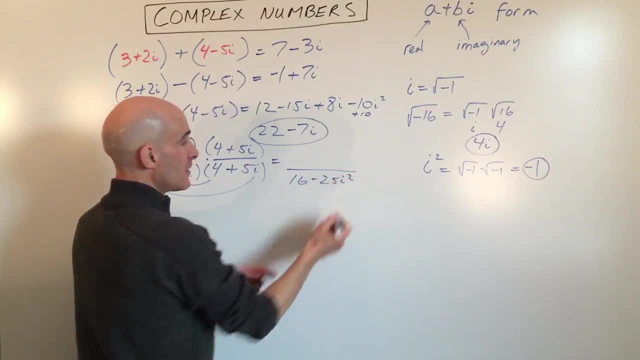 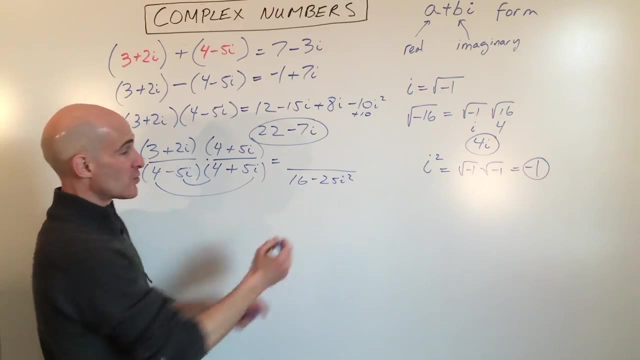 us negative 25i squared. remember i squared is negative 1 times. a negative is a positive, so this is going to be 16i squared. so we're going to multiply these by 16 plus 25, which equals 41 in the numerator. we're going to do the foil. we. 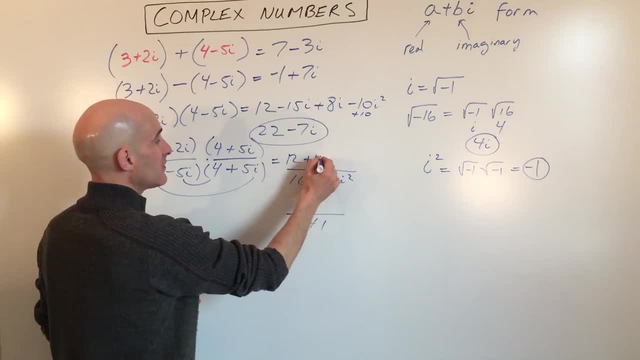 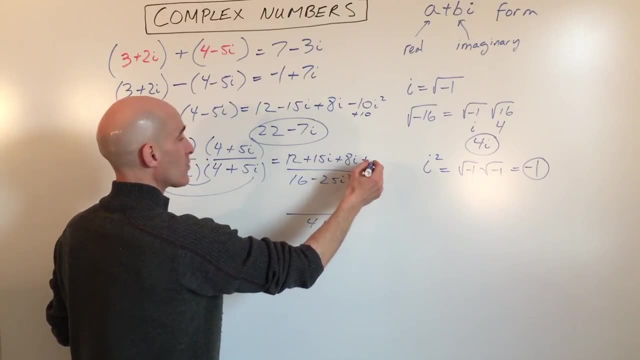 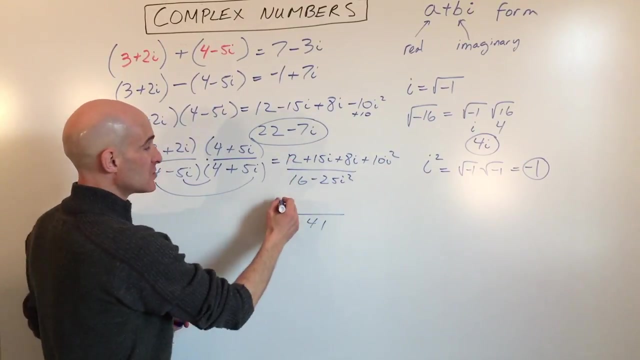 get 12. outer gives us 15i, inner gives us 8i. and the last terms give us 10i. squared. remember i squared is negative 1, so this is actually negative. 10 plus 12 is 2, 15i and 8i gives us 23i. and now here's the part that sometimes students 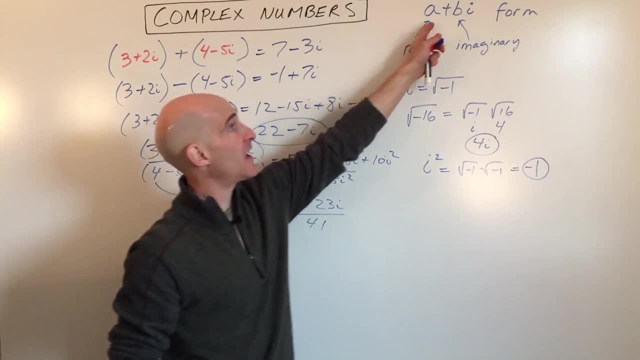 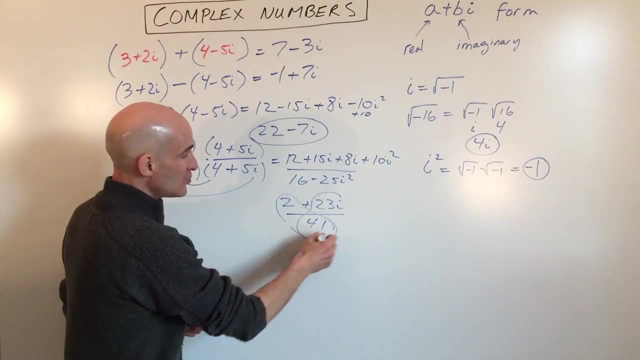 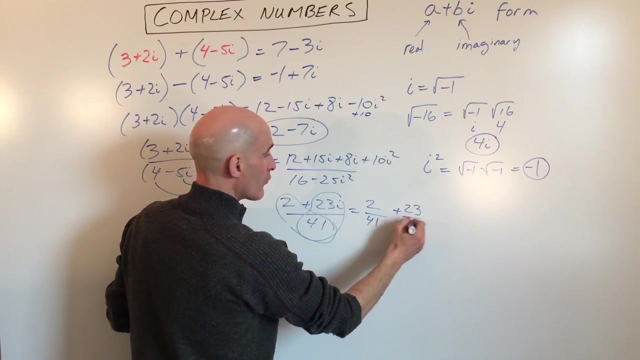 forget looks like we're done, but we actually want to write this in a plus bi form. we want to separate the real and the imaginary part. so the way you do that is, you split this up into two fractions. okay, so this is going to be 2 over 41 plus 23 over 41 i, so there's the real part and there's the 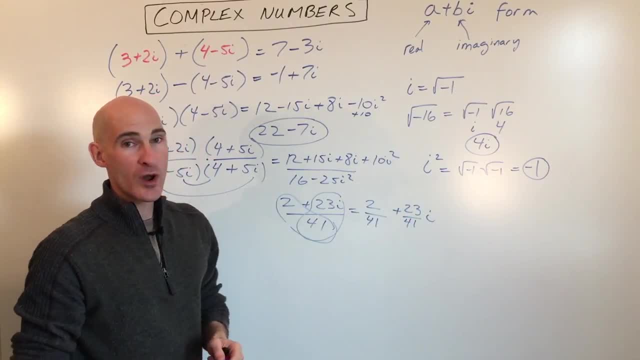 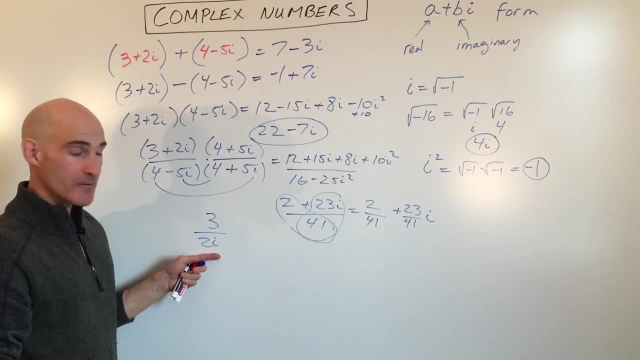 imaginary part a plus bi form. i'll show you one other example real quick. say you just have 3 divided by 2i. this is just a monomial in the denominator, just one term. so what you're going to do here is you're just going to multiply by i over i. this will give you 2i squared, which is: 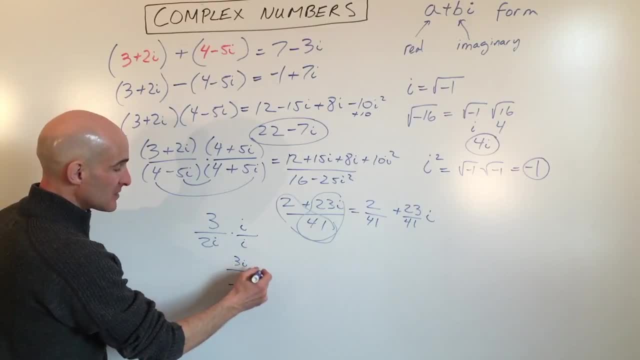 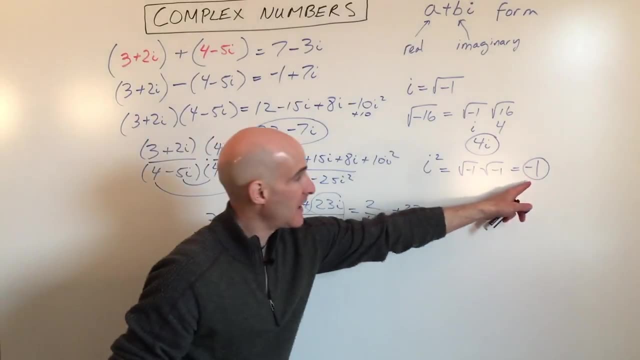 negative 2 and this will give you 3i, so you can just write this as negative three halves i. so again, i times, i gives you the i squared, which is negative one times two, which is negative two, and we just multiply the numerators. whatever you do to the denominator you want to do to.